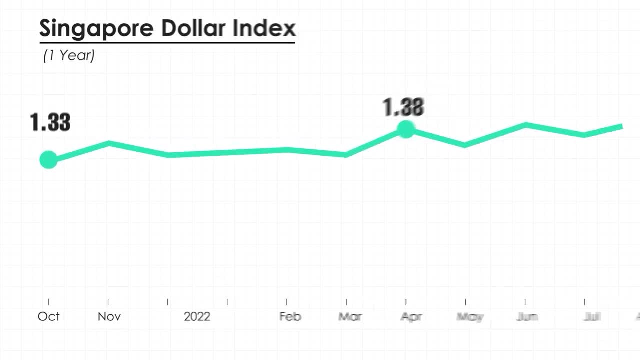 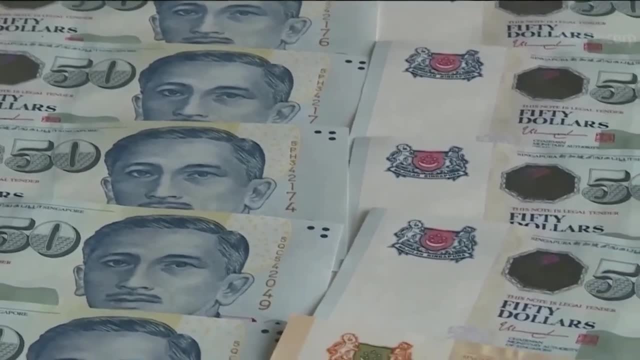 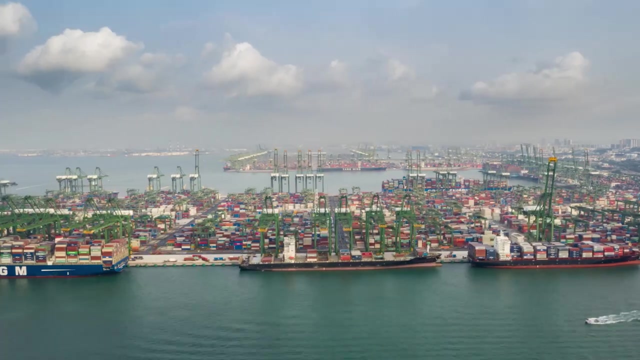 would buy 1.33 Singapore dollars, while in October of the current year, 1.44.. Such results make SGD a regional leader currency that preserved its value. The reason commentators are amazed by the resilience of the SGD is that Singapore is highly dependent on imports. In 2021, Singapore's total trade turnover was 1.1 trillion SGD. 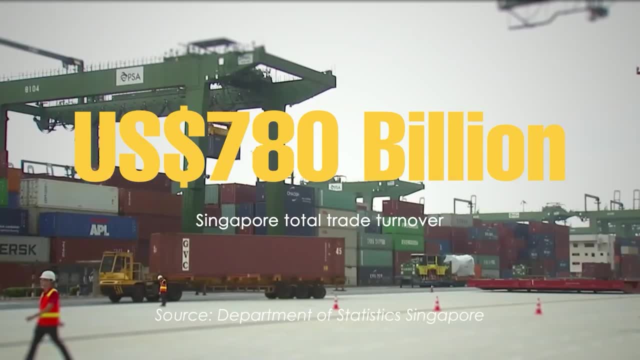 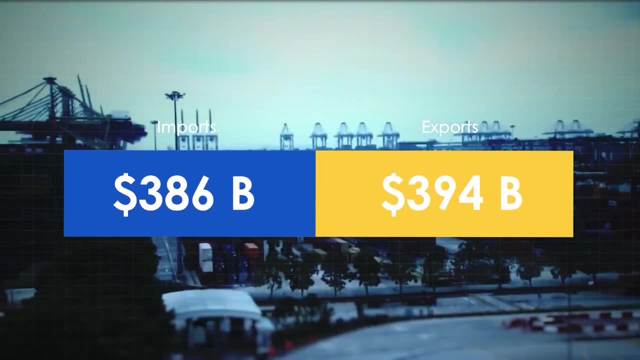 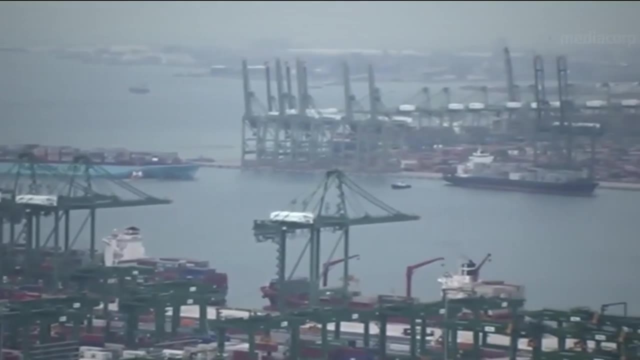 or 780 billion US dollars. Import takes a sizeable share: 545 billion SGD or around 386 billion US dollars. Once again, if Singapore imports over 40% of the goods, how the local currency stays so strong. So let's focus on the current situation. Let's start with the current situation. The 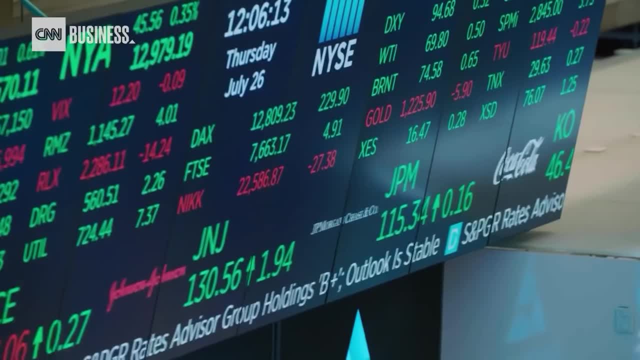 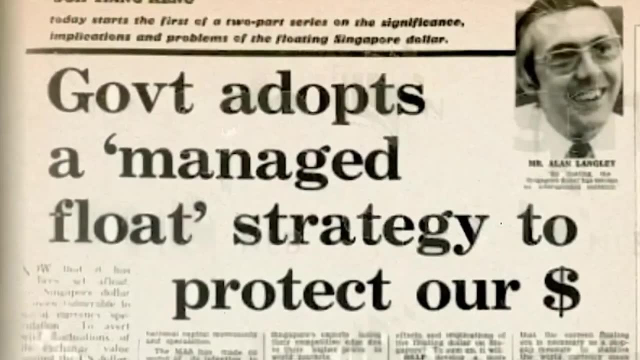 current situation. The current situation. In this regard, Singapore has its know-how. Every country must deal with the exchange rate and intervene in the market. However, since 1981, Singapore has focused on managing the exchange rate instead of interest rates. 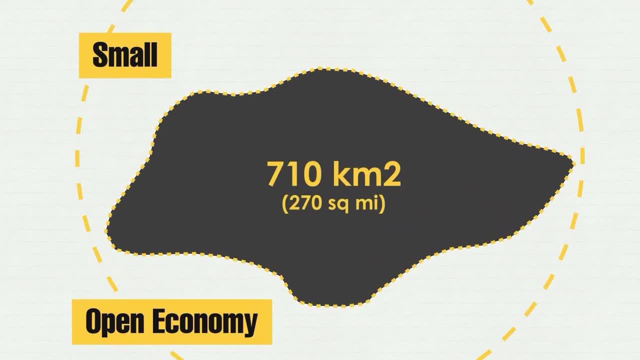 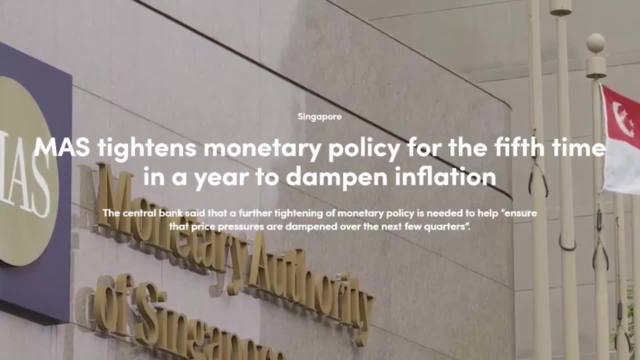 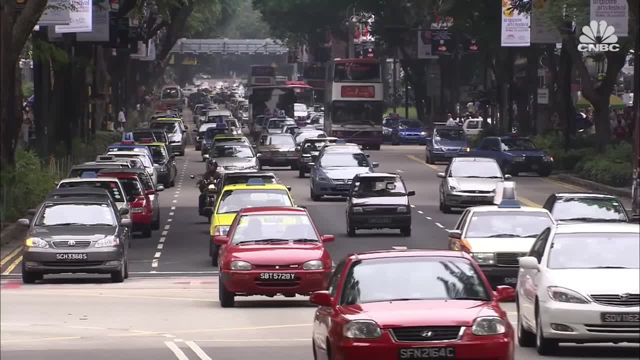 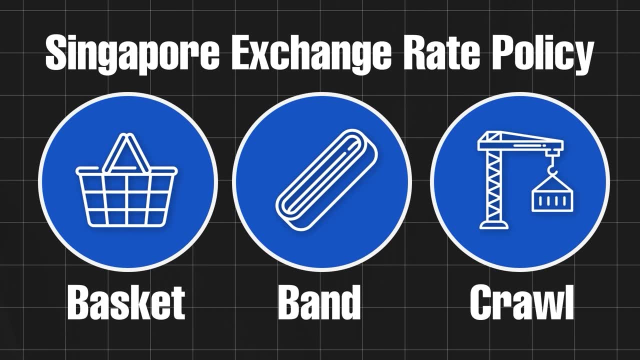 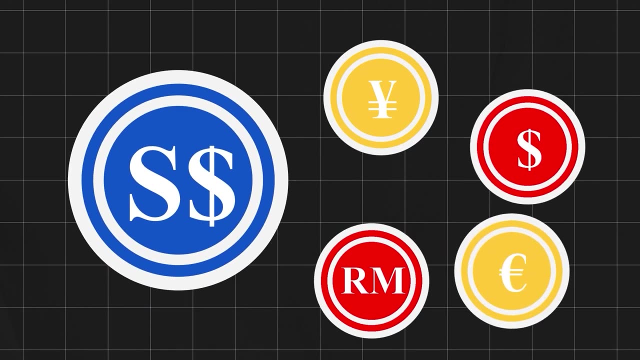 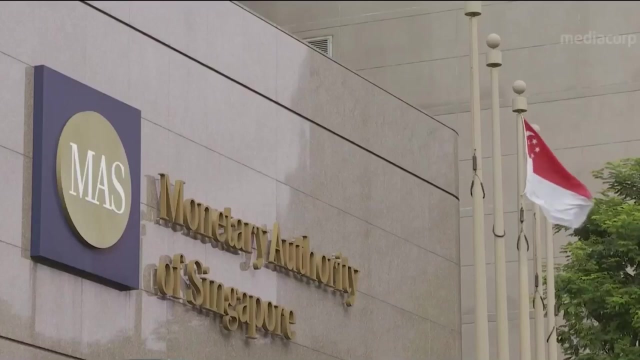 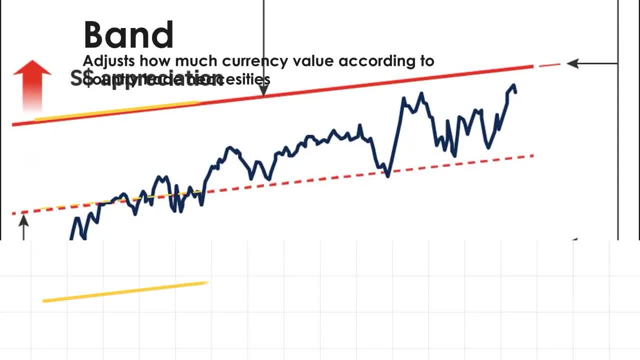 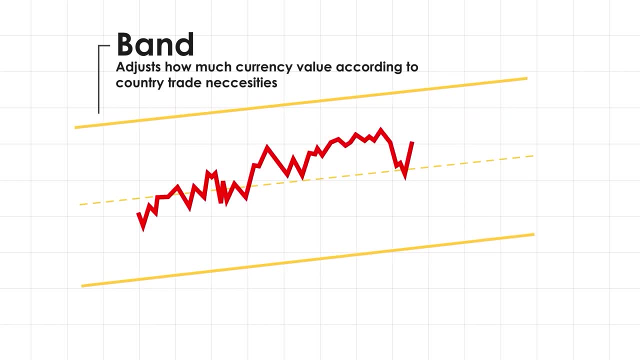 The local currency has a ceiling or a band within which it is allowed to fluctuate. However, one should note that the exchange rate is trade-weighted. Thus, interventions are made according to the country's trade necessities. This mechanism proved to be flexible enough. 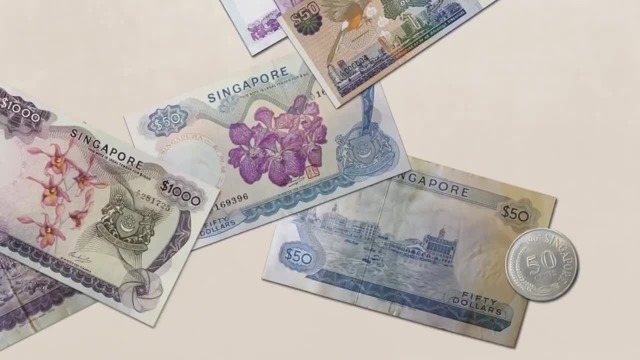 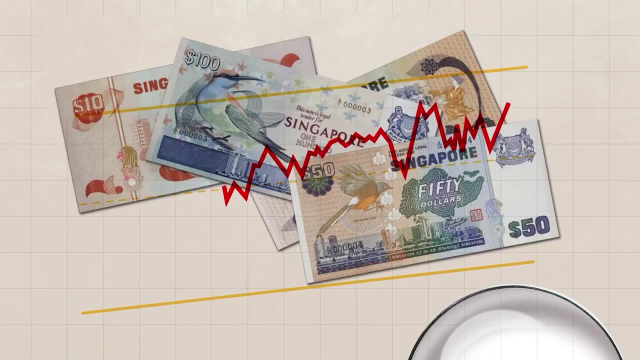 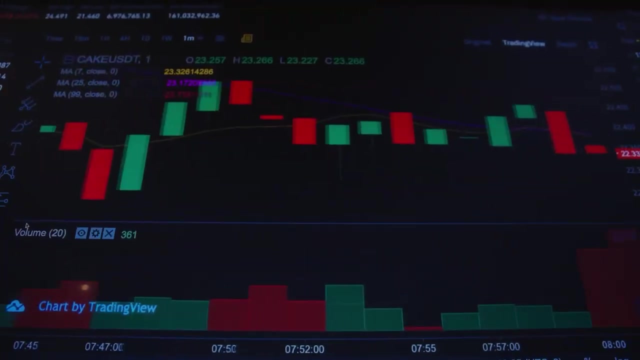 to decrease the need for constant foreign exchange interventions. Third, the crawling system means that the exchange rate policy band is reviewed regularly to keep up with economic trends. In other words, Singapore's authorities can quickly adapt to upcoming financial risks and keep SGD competitive towards major trading currencies. Historically, the Monetary Authority of Singapore has a long record of preventing the internationalisation of SGD. However, as time passed and Singapore became one of the world's financial centres, radical changes were needed. Therefore, in the 1970s, restrictions were gradually removed. 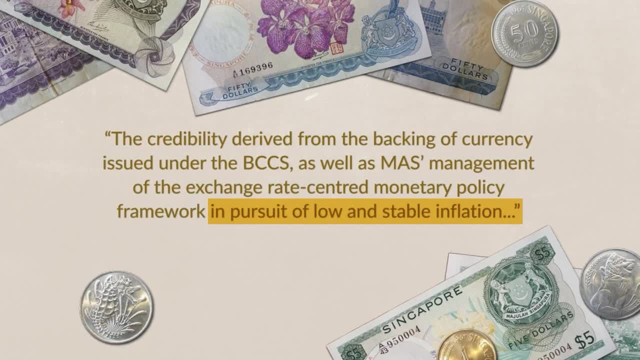 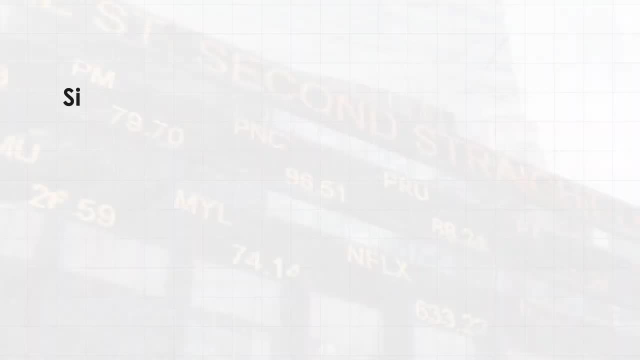 although this policy was beneficial for Singapore, as it maintained inflation low and protected the local currency against speculations, The IMF at the time said the following about Singapore's monetary policy: Singapore's success in maintaining internal and external balance also owed much to the Singapore government's steadfast pursuit. 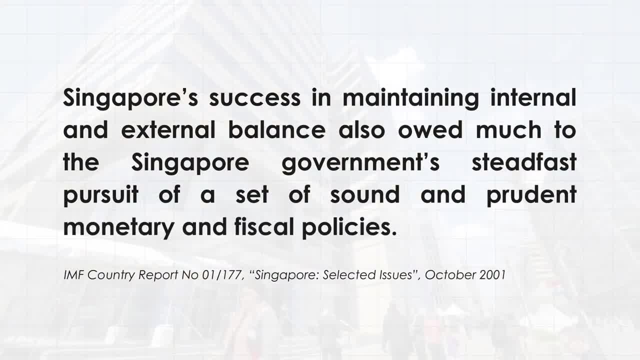 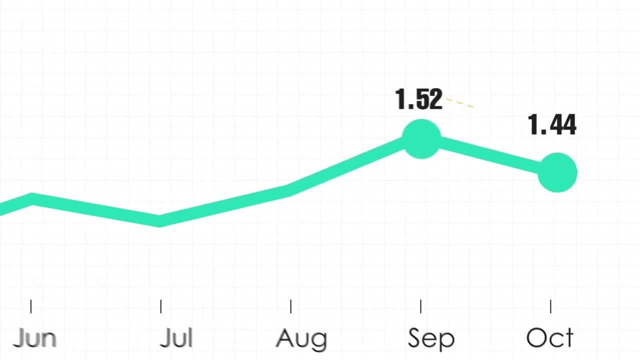 of a set of sound and prudent monetary and fiscal policies. On a practical level, one can see how this system works. For example, in October of the current year, SGD lost its value against the US dollar by 5.7%, outperforming regional peers. 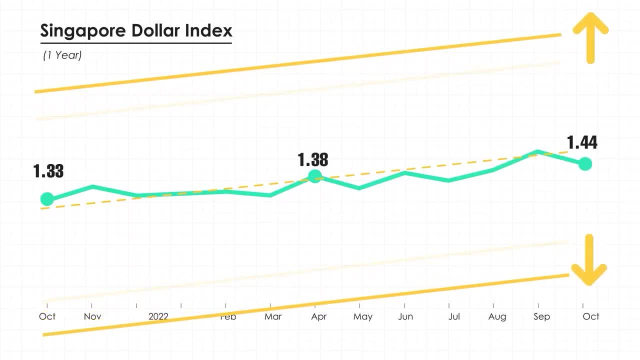 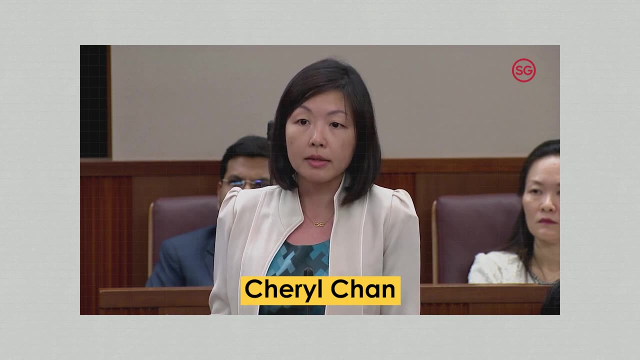 According to MAS, it would raise the band mildly, which is a less invasive strategy than observers anticipated. Cheryl Chan, Senior Vice President for Capital Markets at Digital Securities Exchange ADDX, said By not changing the slope of the band, the MAS took the calibrated approach. of not allowing the pace of currency appreciation to quicken further. This is especially given the fact that the Singapore dollar is already one of the strongest performing currencies against the US dollar so far this year. The more I research this topic, the more I understand that it is the economic system of Singapore as a whole. 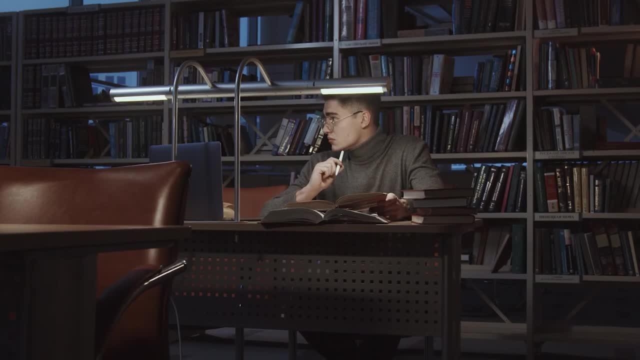 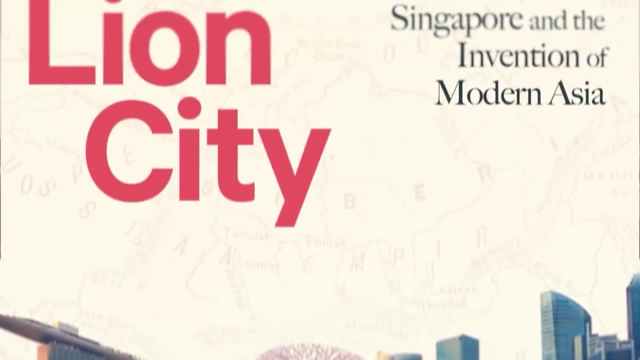 that gives the ability for the currency to stabilise while neighbouring countries struggle. In this respect, one may find the new book of investigative journalist Jeevan Vasagar interesting. His book Lion City, Singapore and the Invention of Modern Asia explains how such a small nation built one of the wealthiest countries in the world. 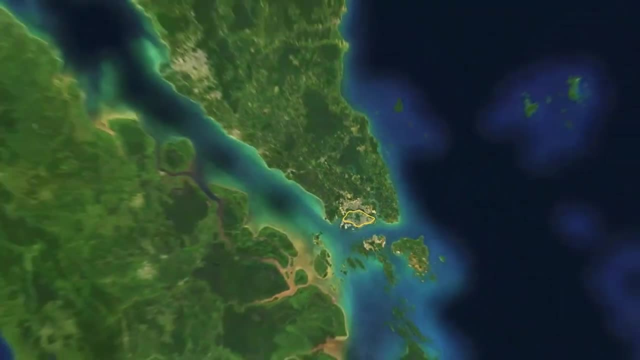 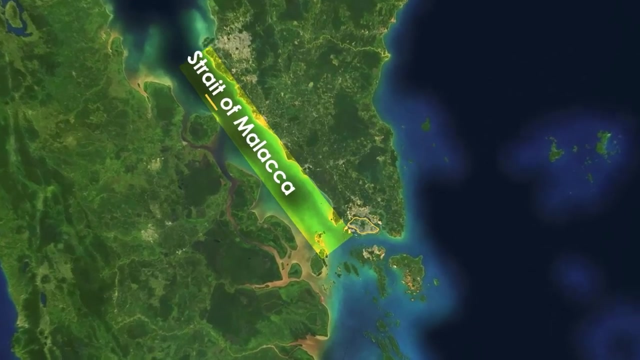 Vasagar mentions Singapore's geographical location as one of the reasons for its economic success. Singapore has to its west a Strait of Malacca which, according to the US Energy Information Administration, in 2015, the Strait was a transit destination for over 60% of the world's petroleum and other energy resources. 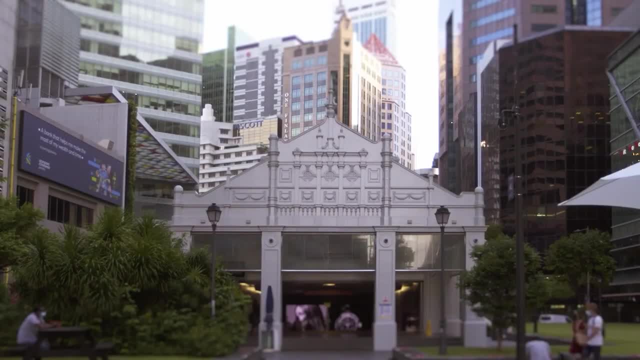 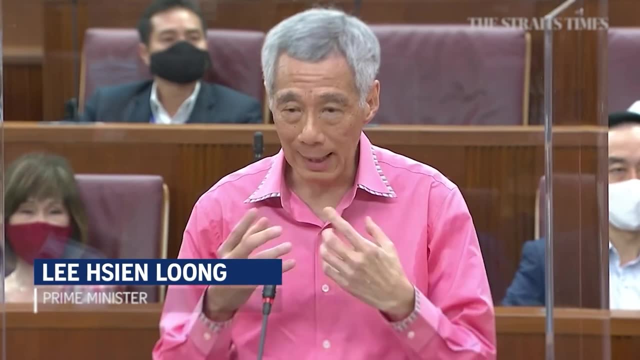 He also adds that, despite such a brilliant location, the most important contributor to Singapore's success is the human factor and sound policymaking. The country's leaders have built a rigorous system that benefited due to its legalistic nature. In addition, according to Gideon Rackman, 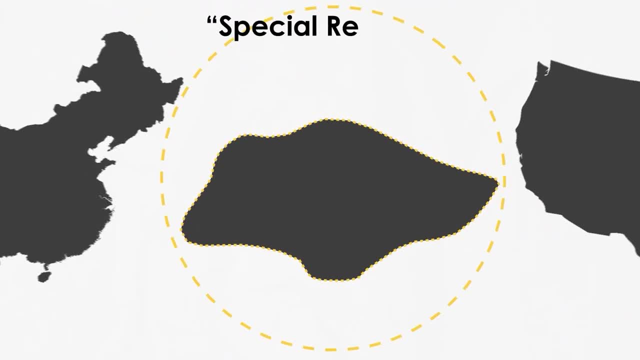 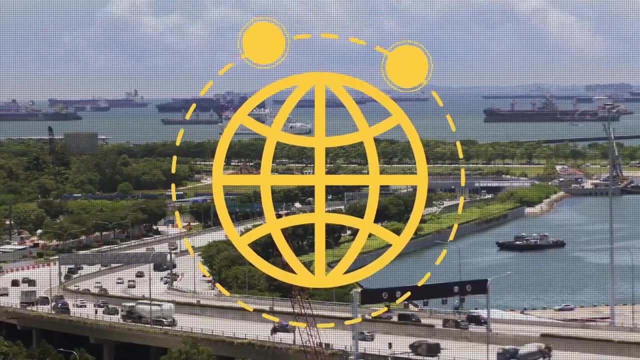 a journalist for the Financial Times. Singapore is the only state with special relations to China and the US. Apart from the above-mentioned reasons, other issues strengthen Singapore's economy. For instance, Singapore has over 20 free trade agreements and over 80 avoidance of debt. 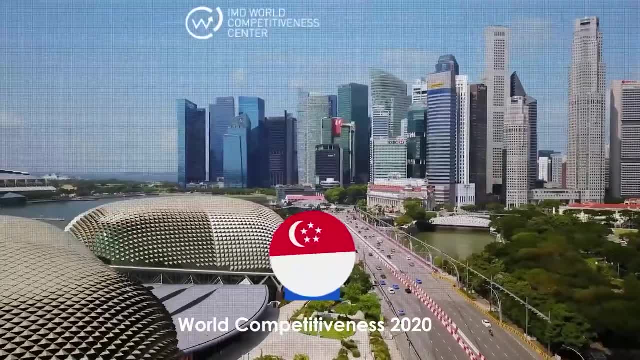 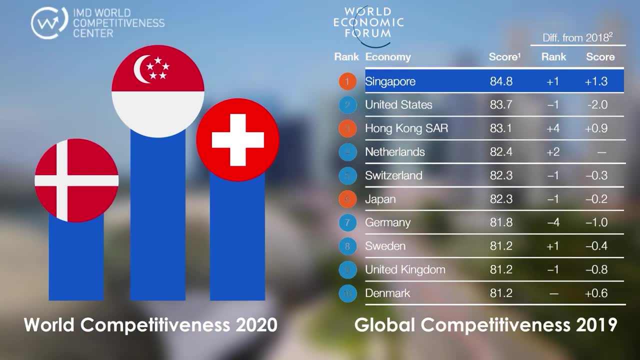 Singapore's global taxation agreements to make the economy attractive. Also, the country was the leader of both IMD's World Competitiveness 2020 and World Economic Forum's Global Competitiveness rankings in 2019.. And according to the 2020, 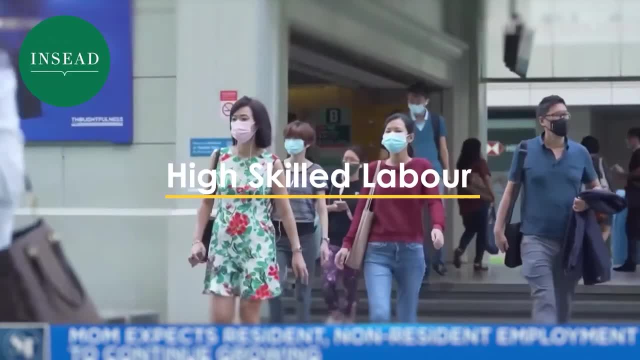 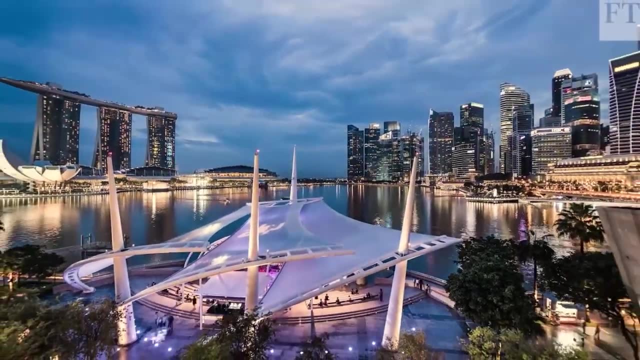 INSEAD Global Talent Competitiveness Index, it has a highly skilled labor force, ranking first in Asia-Pacific and third globally. Furthermore, Singapore will improve its position as a global financial hub. According to the Global Wealth Report, 2022, Hong Kong will replace Switzerland. 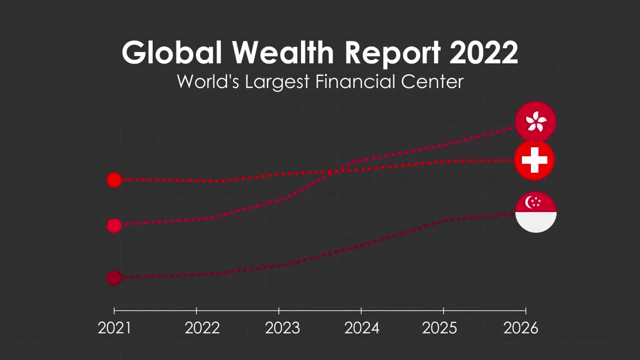 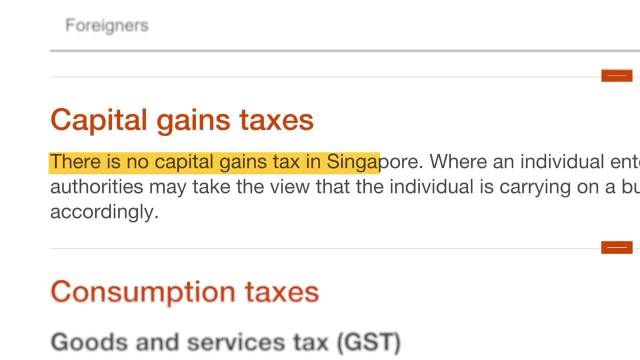 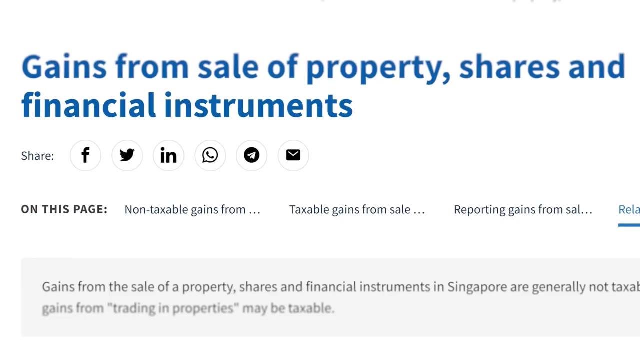 as the world's largest financial center by 2026, and Singapore is coming close to dislodging Switzerland from second place. Besides, Singapore indeed has no capital gains tax. This allows for attracting more investments. However, there is one caveat: If the primary objective of buying and selling shares 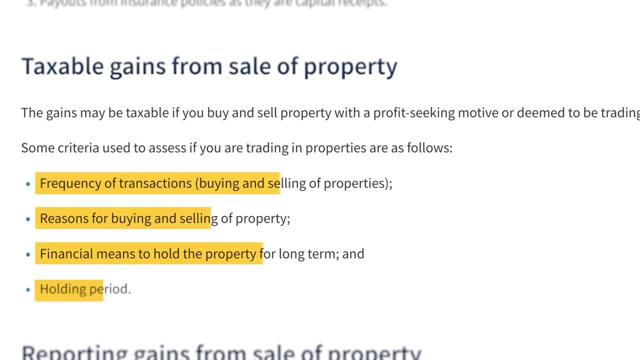 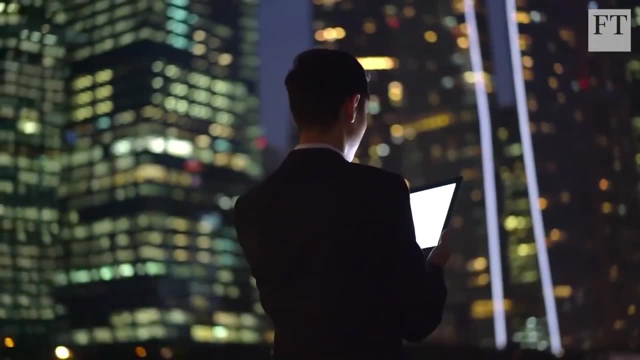 properties and other intangible assets is to make a profit. basically, then, tax on capital gains will be applied. Plus, there is a reason why Singapore is given a triple A score when it comes to credit ratings. However, some economists were concerned with 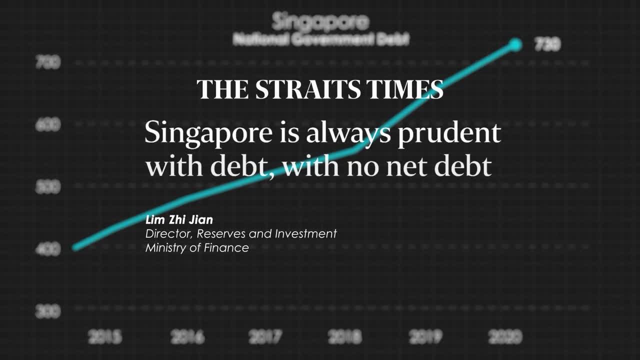 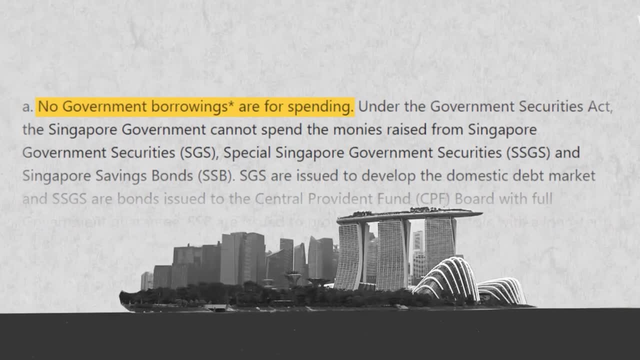 Singapore's high gross national debt and, when examined, experts found that the country has zero net national debt. Lion City's government explained that it is because they do not spend the borrowings and that Singapore is a net creditor country, not a debtor country. 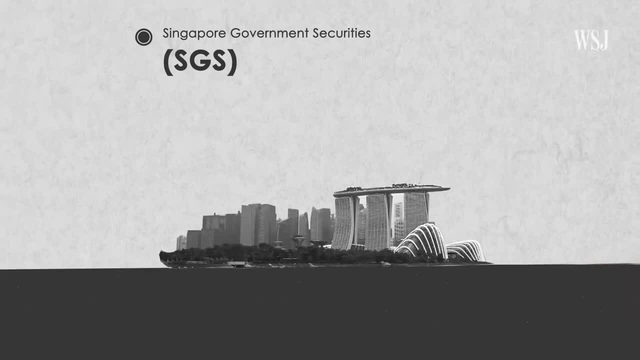 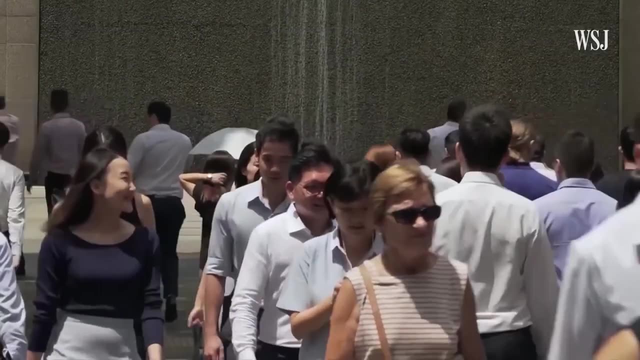 All the credits go through Singapore Government Securities, SGS, Special Singapore Government Securities, SSGS, and Singapore Savings Bonds, SSB. Lastly, the citizens are familiar with and use modern economic tools like stock markets as they care about the state of the economy. 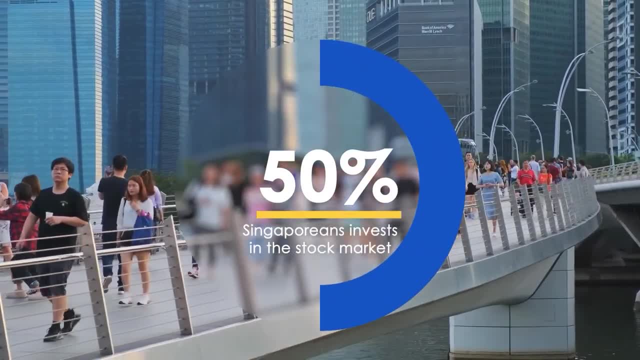 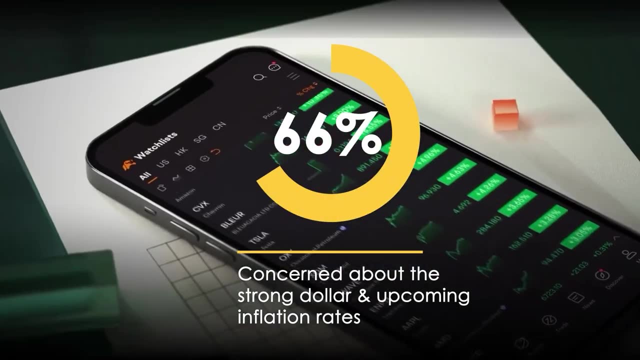 and the country's economy. According to the last year's statistics, 50% of Singaporeans have investments in the stock market And, according to the Moomoo Financial Singapore and Moomoo Wealth Management Platform survey, 66% of the respondents are concerned about the strong dollar. and upcoming inflation rates, and over 80% think that investing is a way to ease the risks of inflation. Overall, Singapore's economy is strong and can prevent significant currency exchange rate fluctuations, as the monetary and fiscal policies of the country prove to be effective.